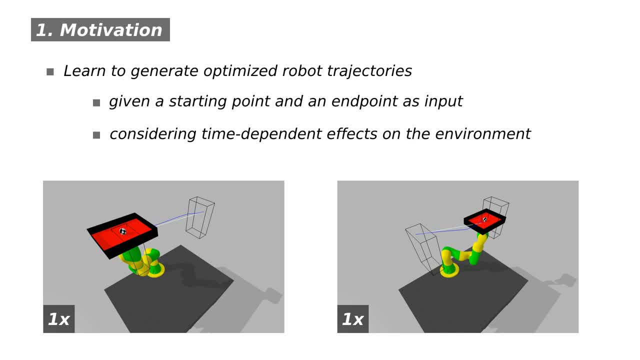 especially if the timing of the trajectory execution is crucial. As an example, consider a robot trying to balance a ball on a plate while moving between specified points. In the videos below, starting points and end points are randomly sampled within the black etched areas, and our goal is to keep the ball as close as possible to the center of the red plate. 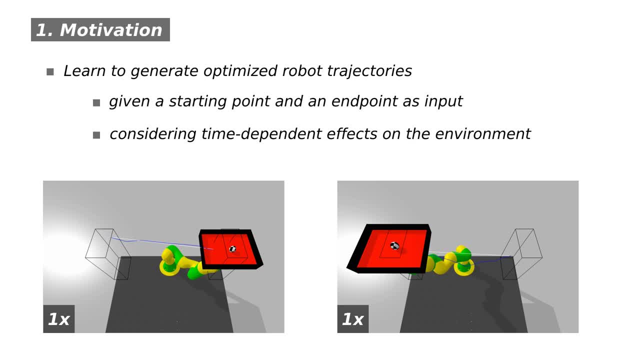 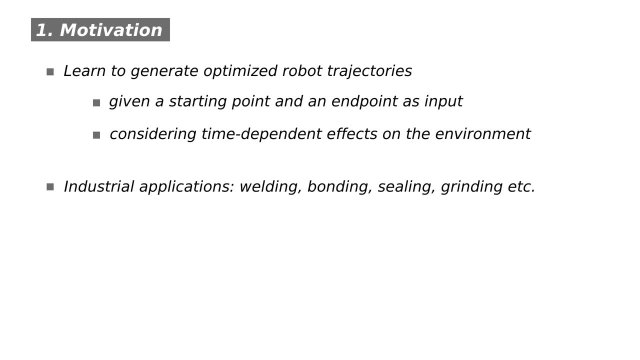 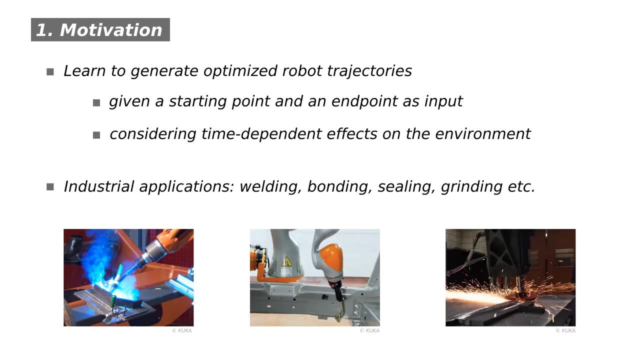 Our question is: can we learn to generate such trajectories from data if we know where the robot should move to and what the robot should do? Problems like this are common in industrial manufacturing. Examples include welding, sealing and grinding. Especially for industrial applications, trajectories are preferred to be: 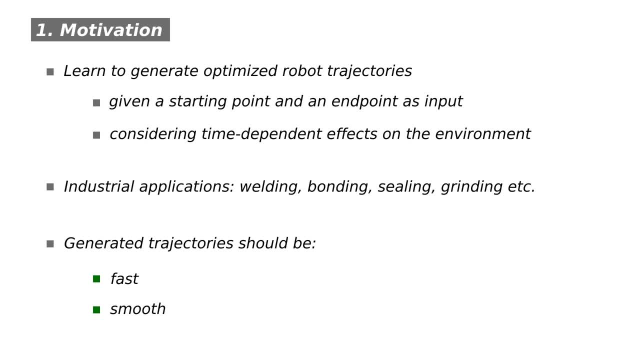 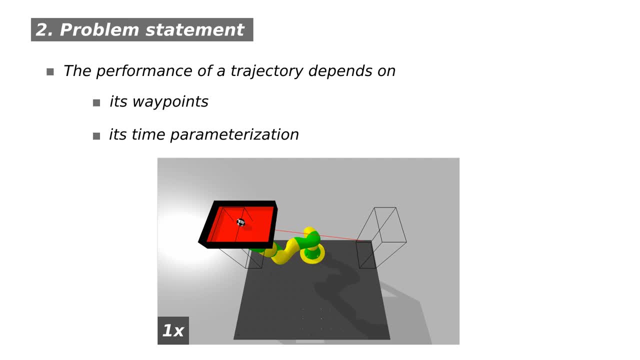 fast and in any case, the generated trajectories should be smooth. Generating good movements for tasks like balancing, welding or grinding is challenging, since the performance of a trajectory depends on both its waypoints and its time parameterization. For instance, when trying to balance a ball, a straight line movement performs poorly, but if we adapt the 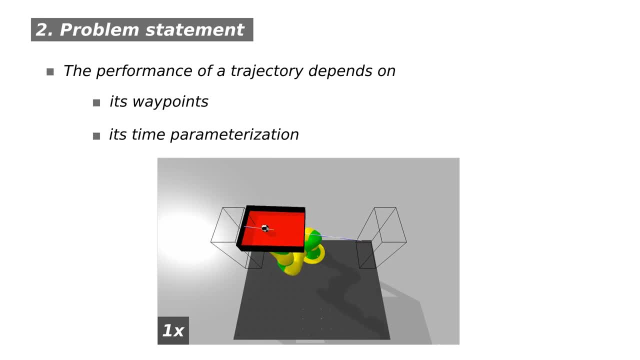 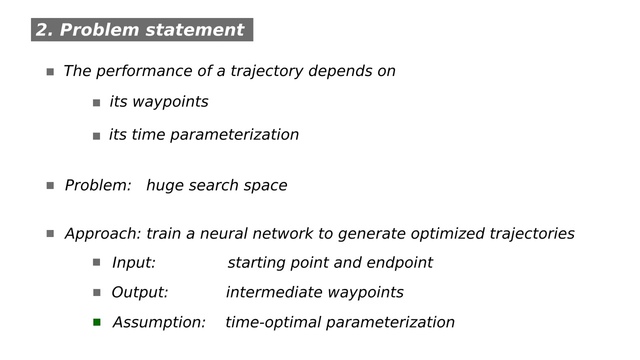 waypoints a little, pretty good results can be achieved. However, if we execute a trajectory with the same waypoints faster or slower, the performance is once again poor. Considering all potential combinations of waypoints and time parameterizations leads to a huge search space. We tackle this problem by assuming that all trajectories 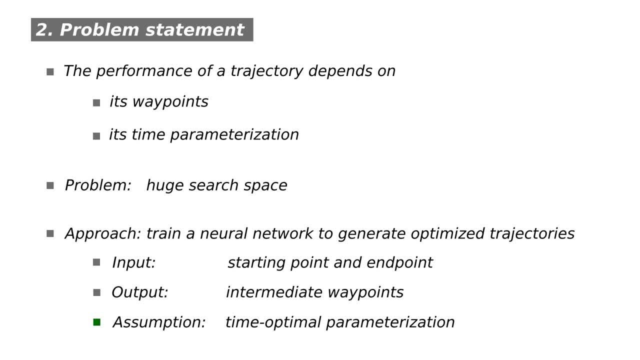 are parameterized in a time-optimal way. Given a starting point and an end point of a trajectory, a neural network is trained to predict intermediate waypoints. Due to our assumption, a unique time parameterization can be assigned to each generated trajectory part. 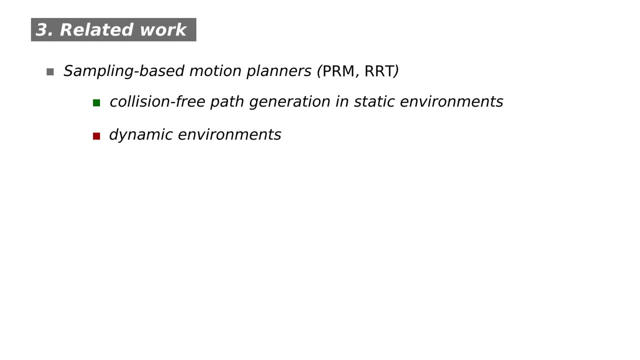 Talking about related work, collision-free trajectories in non-moving environments are typically generated by sampling-based motion planners like PRM or RRT. If timing matters, optimization-based planners like STOMP can be applied. In contrast to our work, STOMP doesn't reuse the experience and the generated trajectories. 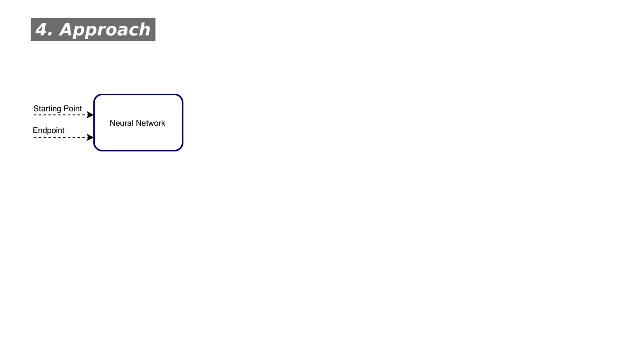 are unparameterized in a time-optimal way. In our approach, the desired starting point and end point of a trajectory are generated by sampling-based motion planners like PRM or RRT. The expected values for each vector of the trajectory are given as input to a neural 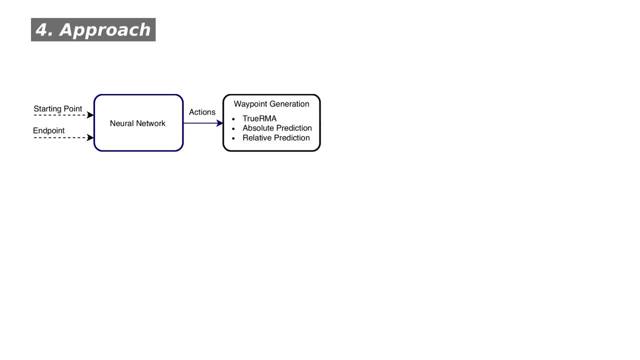 network. The network outputs actions which are used to parametrize intermediate waypoints. We've investigated different techniques for waypoint parameterization which will be explained later. By adding circular planes around the waypoints, a smooth Cartesian path is generated. This Cartesian path is transferred to joint space by an inverse kinematic solver. In effect, Kirchner's different values are assigned to different object types that inform the type of waypoint parameterization. By another way of doing this, the waypoint parameterization is automatically mouseed. Next, at time-optimal time, there are multiple passes which are: 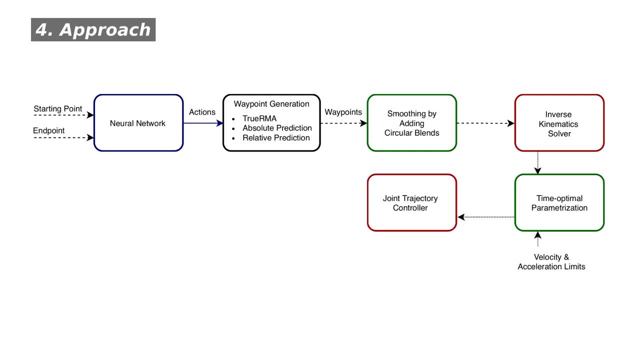 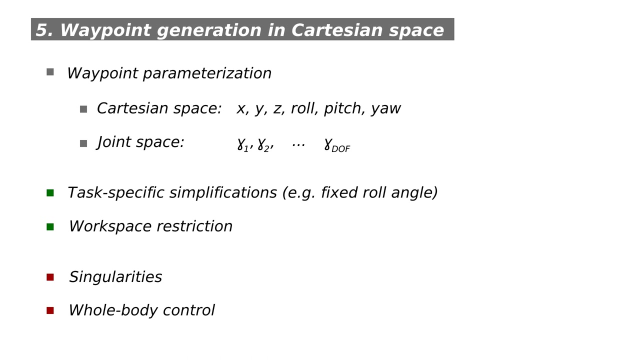 optimization is computed and given to a joint trajectory controller. During training, the trajectory is executed by a physics simulator and its performance is rated with a scalar reward. Using reinforcement learning, the neural network is trained to generate well-performing trajectories. Waypoints can be defined in Cartesian space or in joint space. In Cartesian space, the 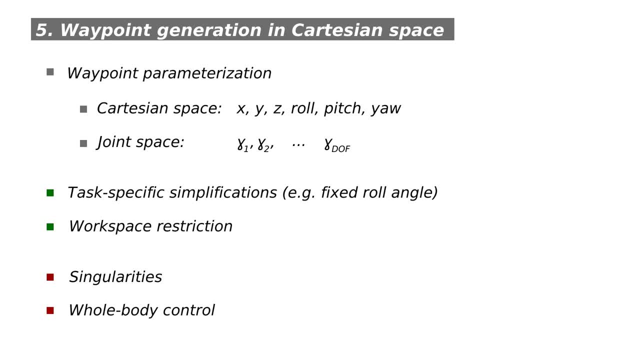 position of the robot's anti-factor is given by values for x, y and z, while the orientation can be specified with roll, pitch and yaw angles. In joint space, a waypoint is defined by one angle per joint When working in Cartesian space. 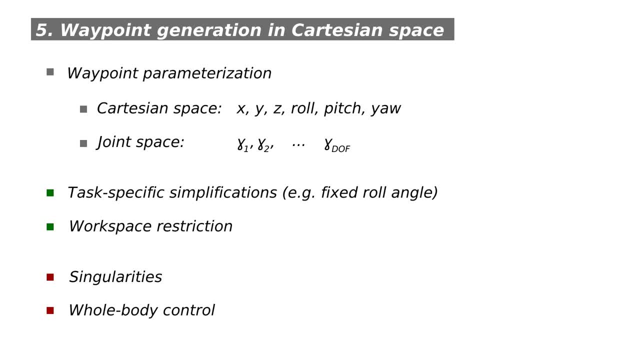 task-specific knowledge can be incorporated. For instance, in our experiments, the roll angle of the balance board is set to a fixed value. Another advantage is that the work space can be easily restricted. On the contrary, special care must be taken to avoid singularities and waypoint. 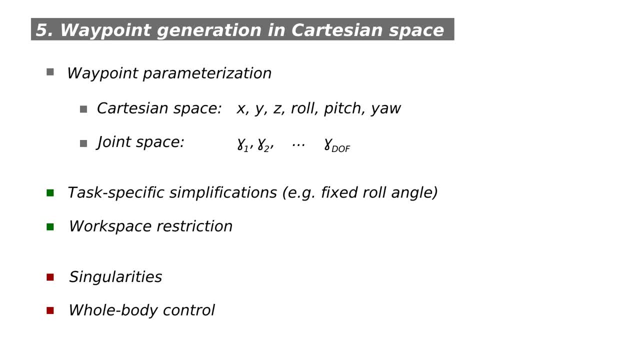 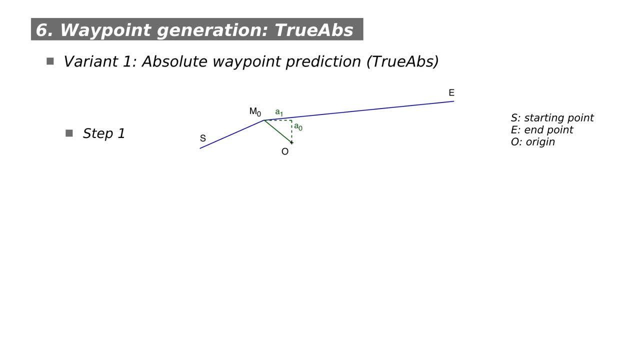 predictions in Cartesian space is not directly applicable to whole body control. The output of a neural network can be directly mapped to intermediate waypoints. In our simplified planar example, the x and y coordinates are predicted for each intermediate point. Thanks for watching waypoint. In a final step, the path is smoothed by adding circular plans With. 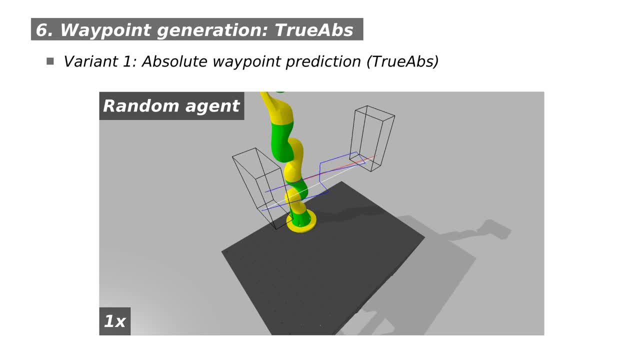 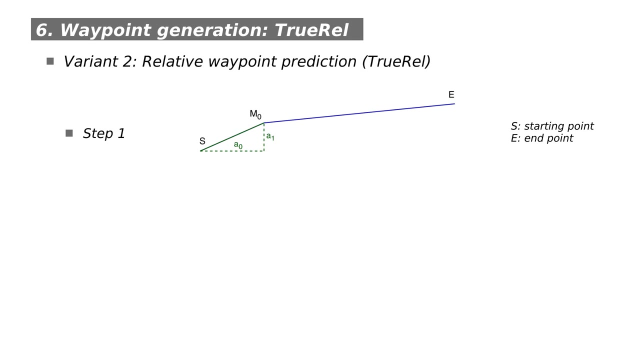 this technique, which we call TrueApps, an untrained agent, generates very long and poorly performing trajectories. It is also possible to define waypoints relative to each other by predicting the deviation to the previous waypoint. Once again, two parameters are required to define a waypoint. in our simplified 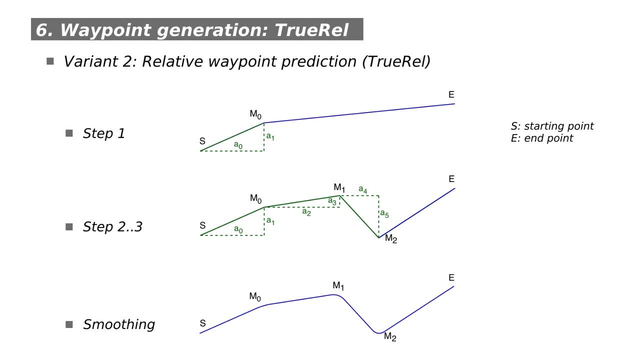 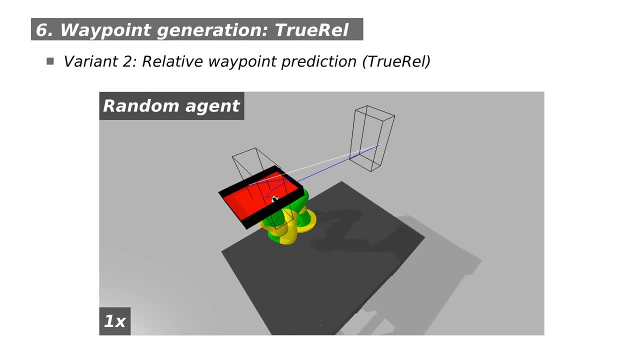 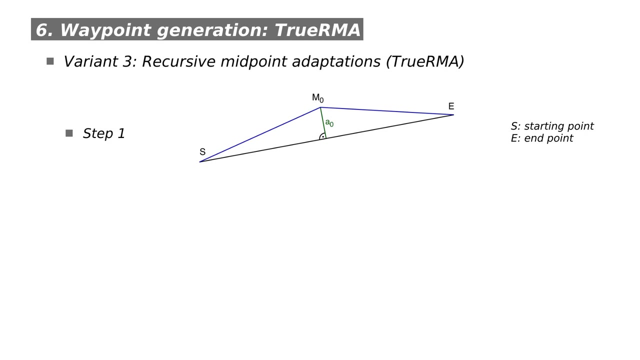 example, A random agent generates waypoints close to the starting point, as the predicted deviations cancel each other. Finally, a path can be defined by recursively predicting orthodoxy. This way, only one parameter per waypoint is required in our simplified example, meaning that the search space of our neural network is narrowed. 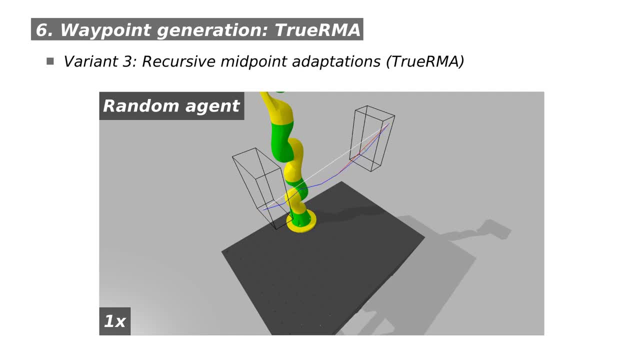 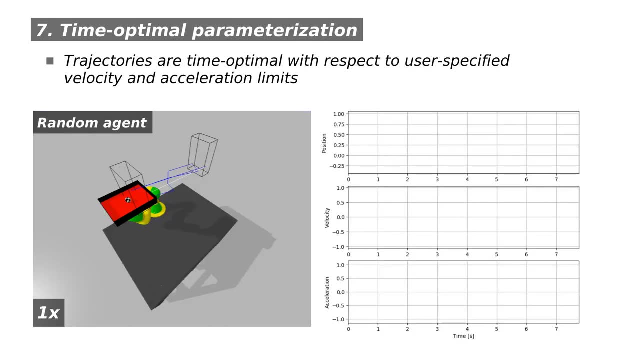 Having a look at a random agent, we can see that the intermediate waypoints are evenly spread between the starting point and end point. Once the path is generated, a time-optimal parameterization is computed. Time-optimality means that at all times, at least one joint is working at its velocity. 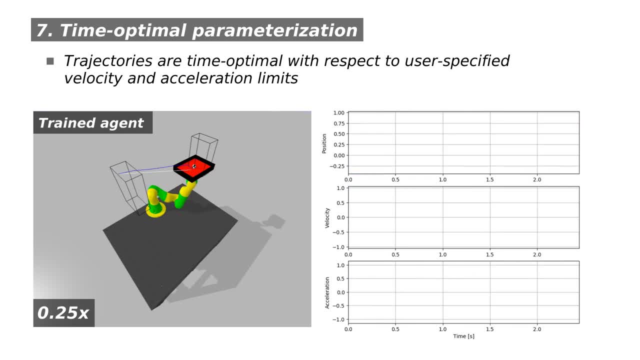 limit or its acceleration limit Close to the starting point and the end point, the execution speed of this exemplary rollout is restricted due to acceleration limits In the intervening time. the maximum velocity of joint 1 is the limiting factor. So the time-optimality of joint 1 is the limiting factor. So let's compare how the presented 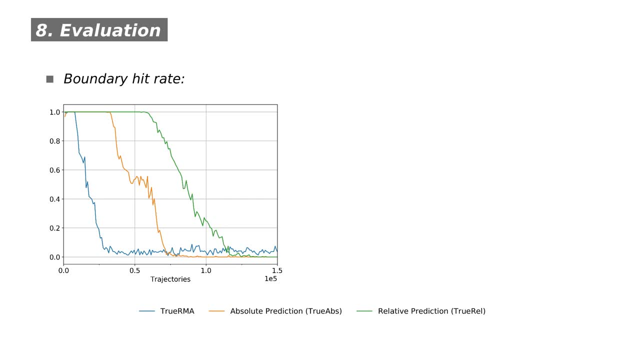 techniques to define waypoints perform during the course of training. We start with the boundary hit rate, meaning the probability that the ball hits the black boundary of the balance board during trajectory execution. Given enough data, all techniques learn to keep the ball on the plate. but true RMA learns significantly faster From a mathematical. 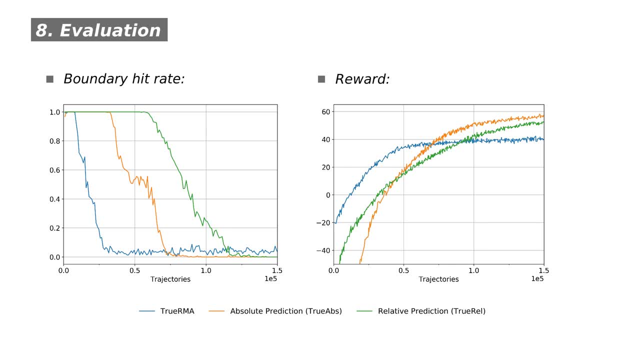 perspective. the goal of the training process is to maximize the number of hits per ball. The goal of the training process is to maximize the number of hits per ball. The goal of the goal of the training process is to maximize the number of hits per ball. The goal of the 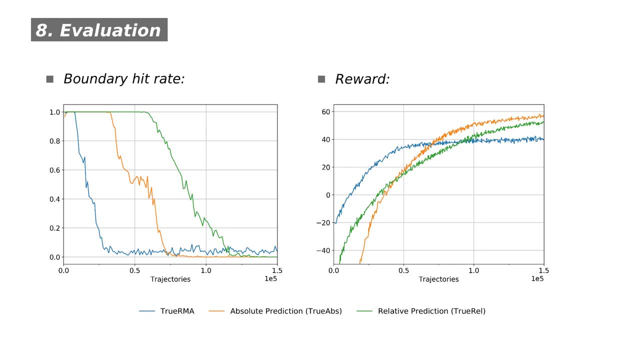 training process is to maximize the average reward. In our experiments, the reward is assigned based on the average distance between the ball and the center of the plate. We can see that the best performance is achieved with absolute waypoint prediction, while true RMA converges against the lower value In this. 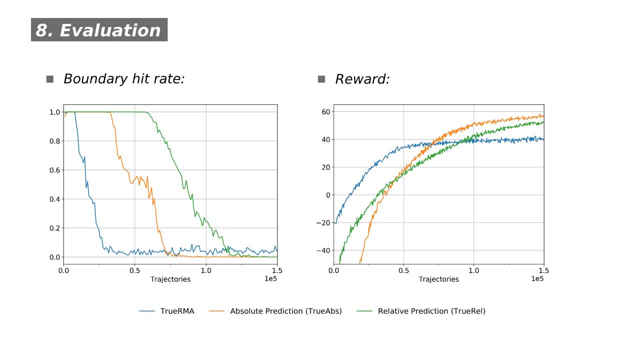 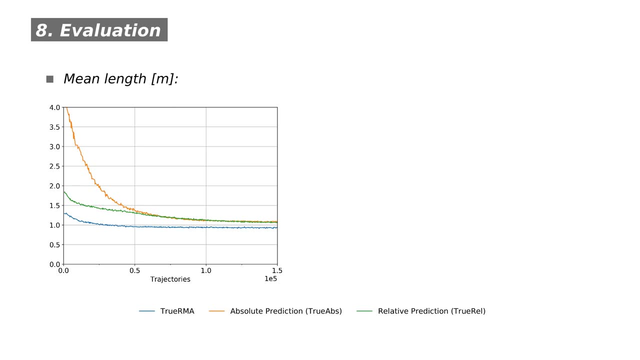 case, the smaller search space of true RMA leads to faster learning at the cost of final performance. As shown in this figure, TrueARM-A produces the shortest trajectories, which is reasonable, as the search is guided by stripline movements. TrueApps starts with very long trajectories, but finally learns to generate short ones.